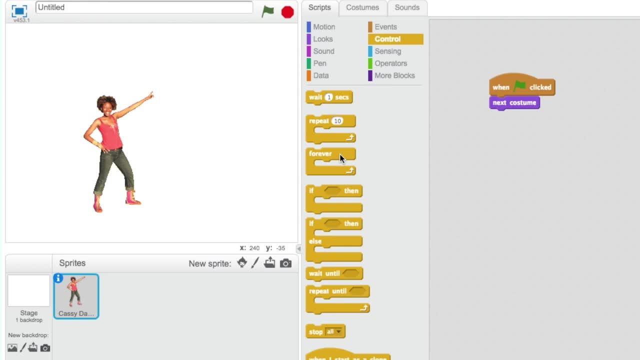 like the forever block is about to eat this block. These blocks should click together. Now the animation is complete, Let's click on the green flag and test the code. It works. Have a look at your sprite. How is the speed of your animation If your sprite is moving? 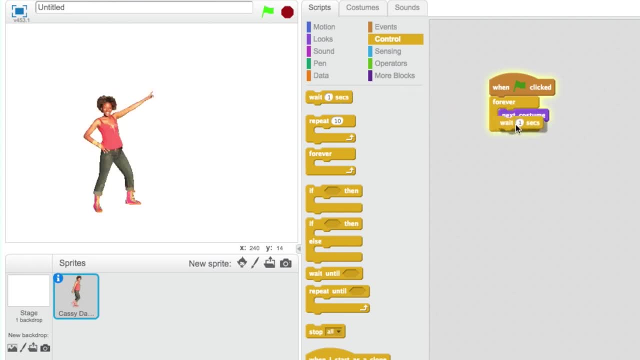 too fast. you can add a weight block found in the control category. By changing the number in the weight block, we can increase and decrease the amount of time between each costume change. For step two, let's paint a new backdrop for our dance party. Click on the miniature. 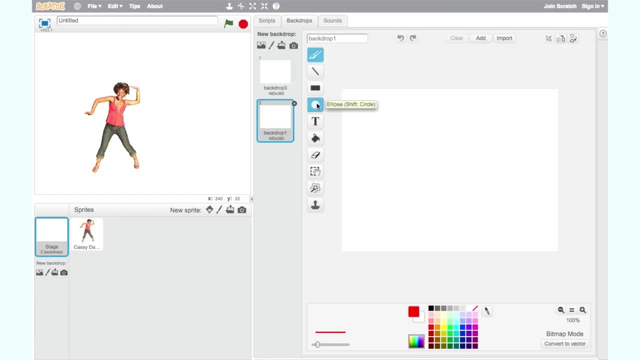 paint new backdrop icon on the bottom left of the screen. You can add different circles with various colours as the colourful lights, and also put some colourful bricks on the bottom of your backdrop by using the rectangle, As we need to change our backdrop during our dance party. we need more costumes for 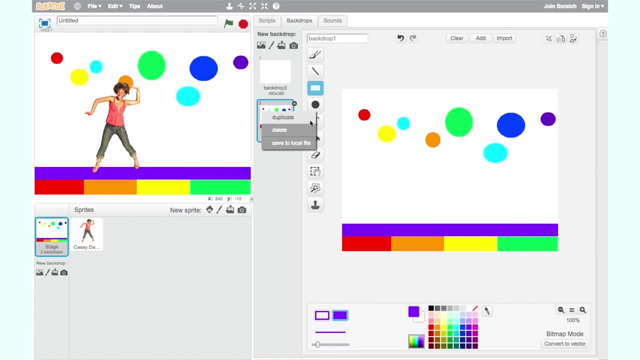 our backdrop. You can right click on your backdrop and select duplicate to copy your first backdrop as many times as you want. Then go to the second backdrop costume and change the colour of each object to different colours. to your first backdrop costume You can use an icon that says fill with colour. 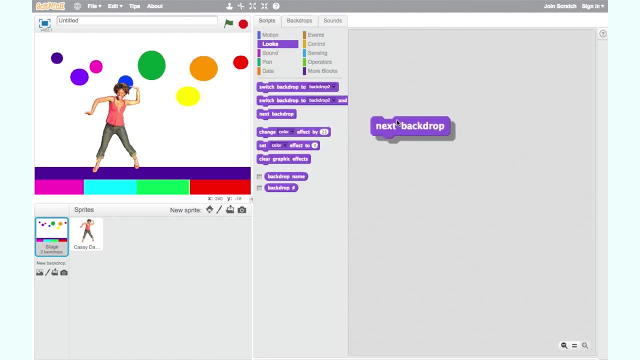 To animate our backdrop, we need a block that says next backdrop, under the looks category and the when green flag clicked block. This will make the lights and dance floor appear to flash different colours. To make our animation repeat forever. we hover a forever loop over. 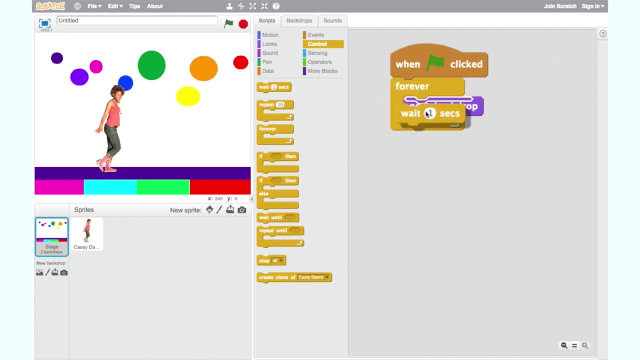 the next backdrop block. To slow it down, we put a weight block after next backdrop. We can change the speed by changing the number to 0.2. For step 3, we want to add sound to our dance party. First we need to get our event block. 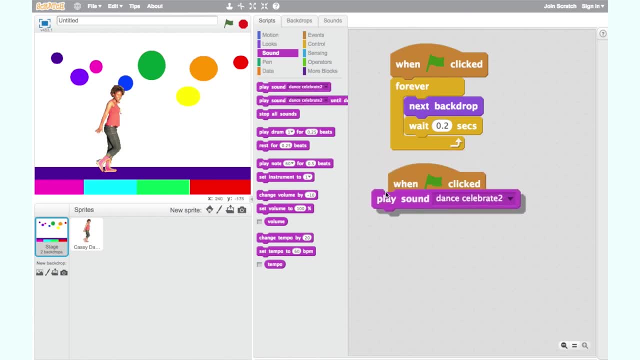 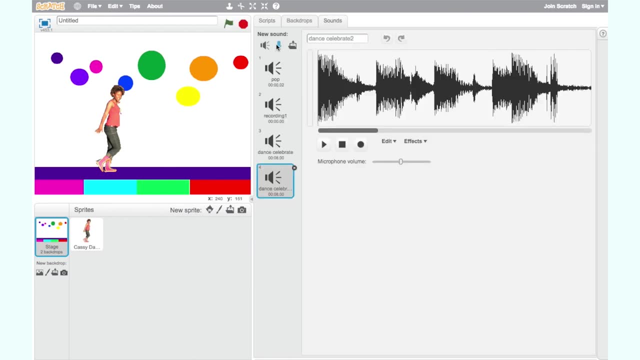 when green flag clicked. Next we want to add a block that says play sound, which can be found under the sound category. To choose the sound that you want, click on the sound header at the top of the screen, Click on the speaker icon and choose a sound you like.